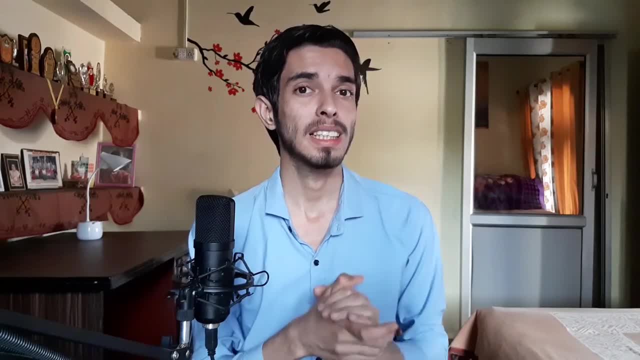 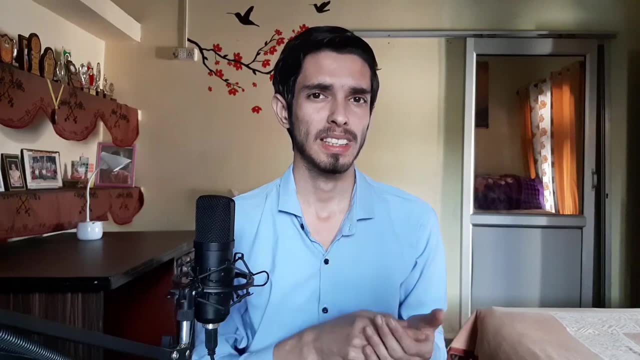 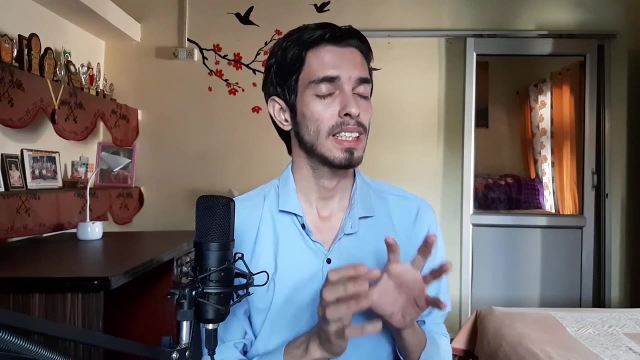 Counting problems are the problems in which the question normally asks in how many ways? And problem like these are literally everywhere, from competitive exams to entrances and in different fields of physics like statistical mechanics. So knowing the number of ways is really important and this makes knowing how to solve counting problems a very essential. 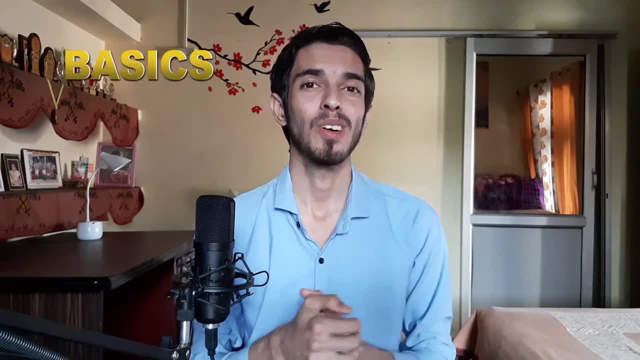 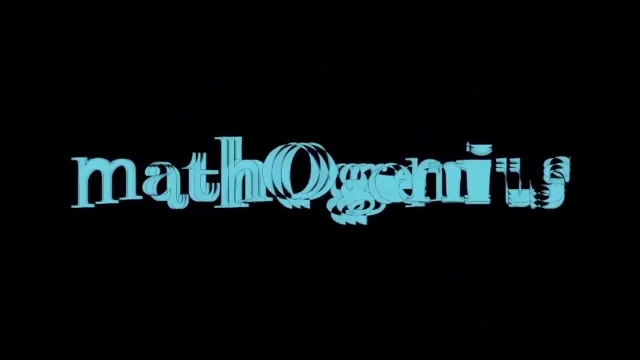 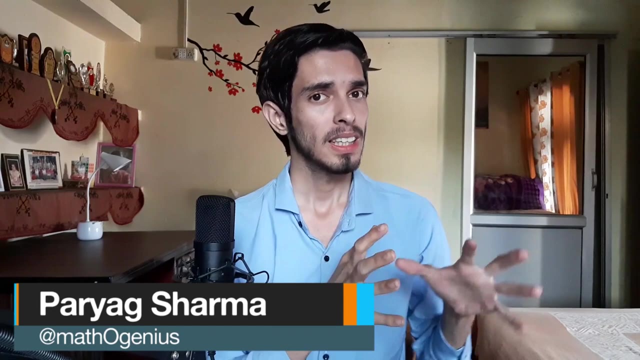 skill to have. So in this video we will learn the basics of counting problems. So let's begin. Hello geniuses, Welcome to this video in MathoGenius Nutshell Math series. In this series, I will make videos related to different topics of math and will teach them to. 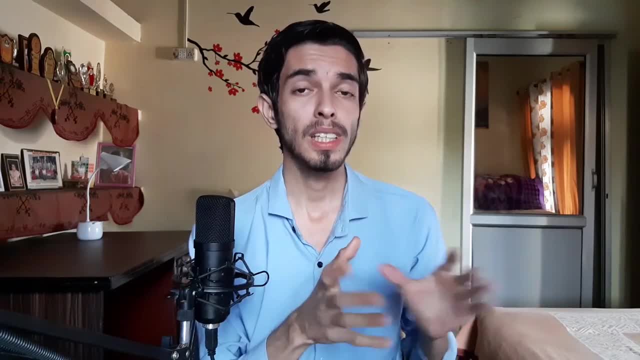 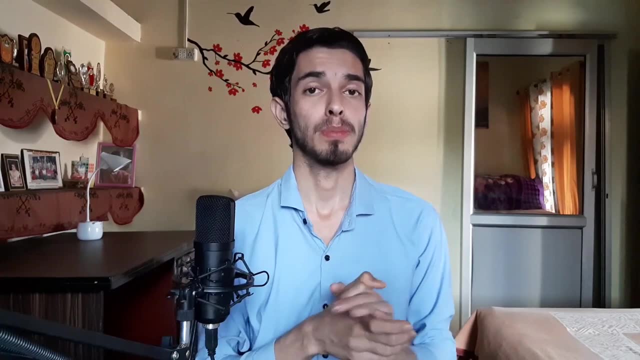 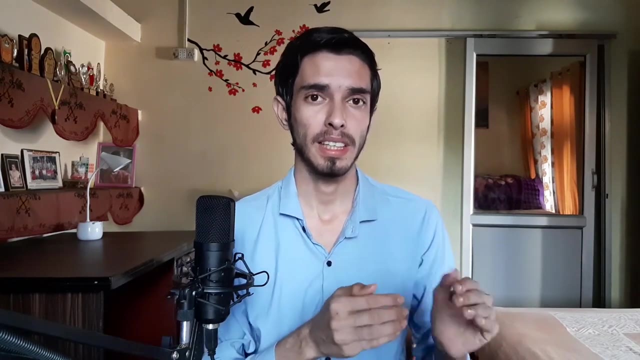 you in a nutshell. So most counting problems boil down to two rules: The rule of sum and the rule of products. These two rules are extremely simple, but being able to identify which one to use is really important, and most of us makes mistake here. So first let's understand the rule of sum. 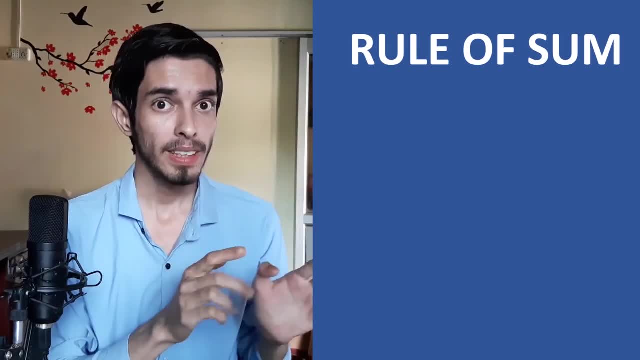 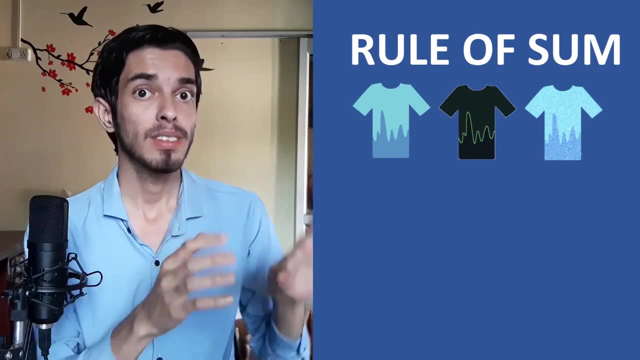 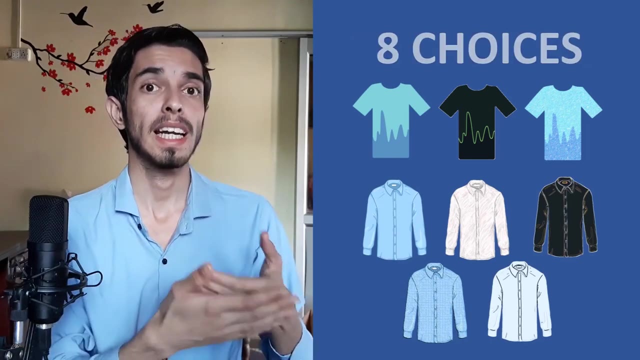 This is used when we need to know the options when we have two separate different choices. For example, you have three different short sleeved shirts and five different long sleeve shirts, Then the number of choices you have are five plus three, which is eight different choices. 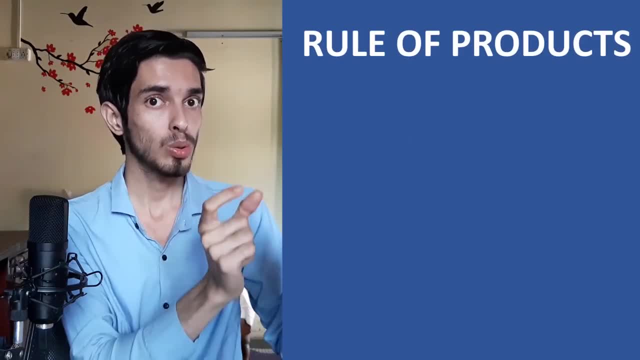 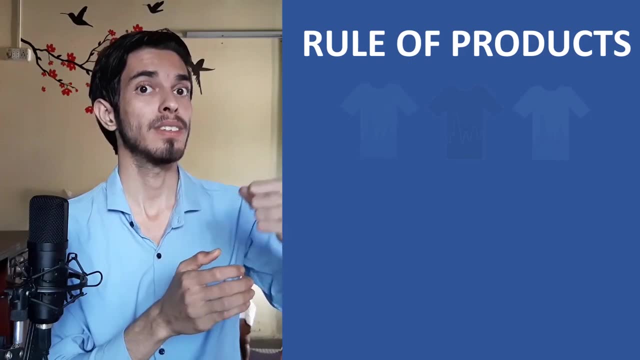 Now the rule of product is used when you have one thing and b ways to do another thing of the same whole thing. For example, you have three different shirts and four different pants, Then the number of ways in which you can wear them is. 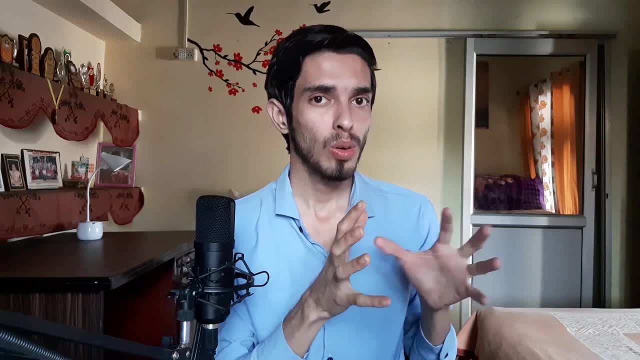 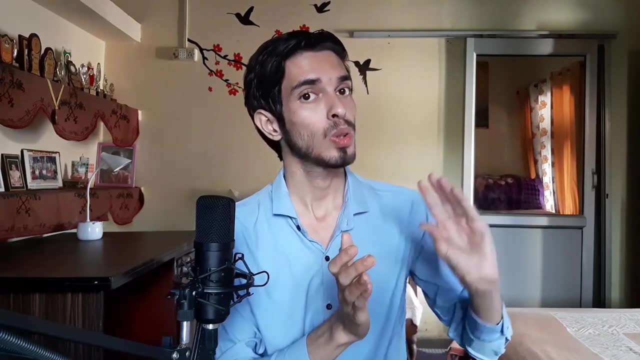 four through the twelve ways. and these twelve ways are only there when you don't have any constraint, like you don't need to match color, etc. etc. These constraints are also there in those questions, So you need to consider these constraints too. So now, what you have learned are really two big keys. 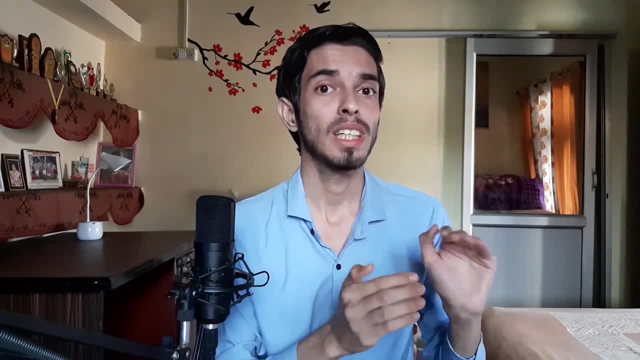 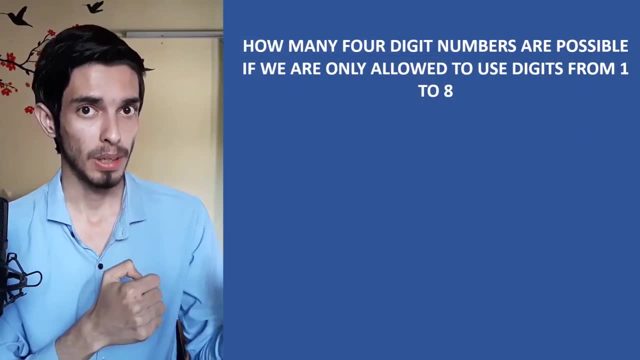 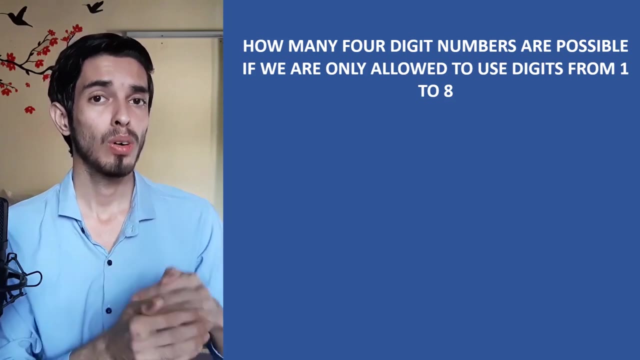 So now let's apply this knowledge to solve a simple counting problem question. The question is how many four digit numbers are possible if we are only allowed to use digits from one to eight? So now try to do it yourself. Use your own common sense and the rule of sum, and 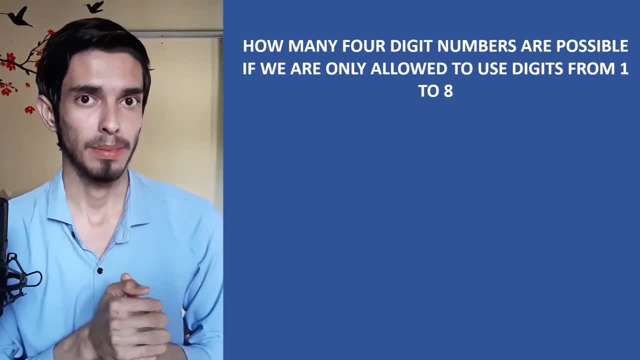 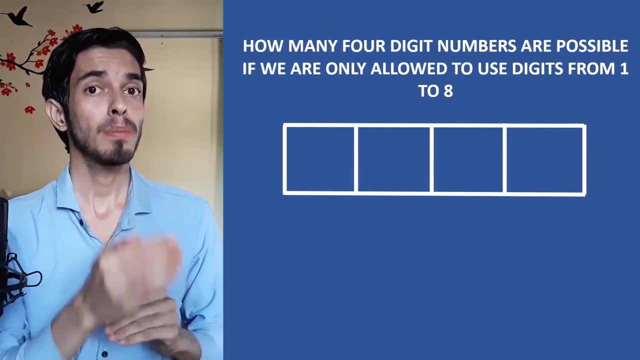 product to find the number of digits. Now, see, it's really simple. See, we have four different slots and we need to choose four different numbers. right Now, the number of ways in which we can choose the first digit is eight. right Now, the number of ways in 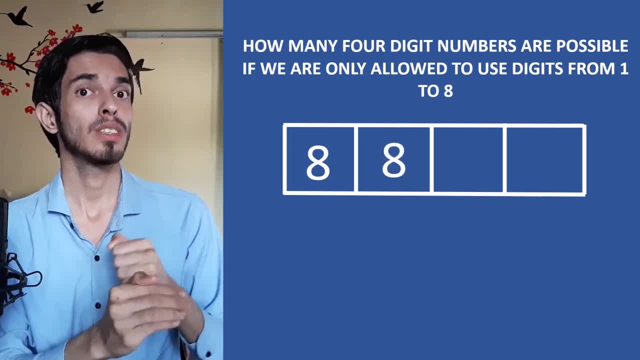 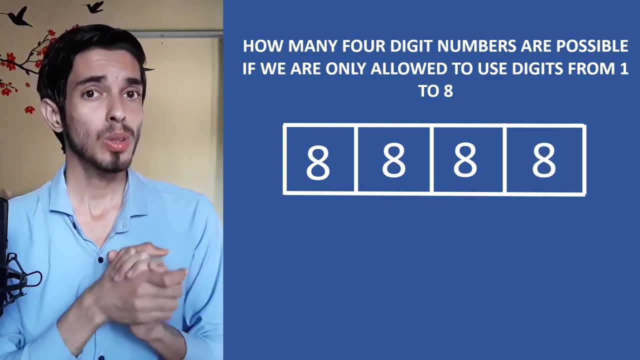 which we choose the second digit is eight. the number of ways in which we can choose the third digit is eight, and the number of ways in which we can choose the fourth digit is eight too. Now, for this whole work to be done, we have a number of ways to do the first part. b number of ways to do. 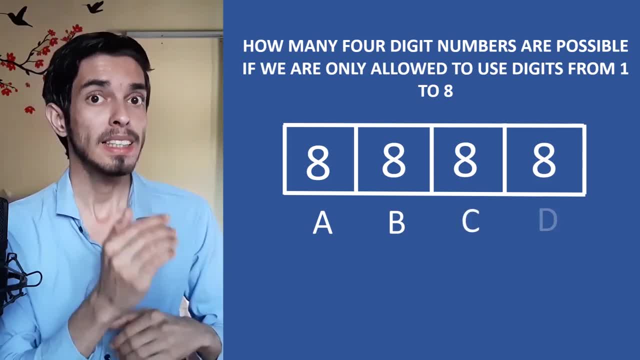 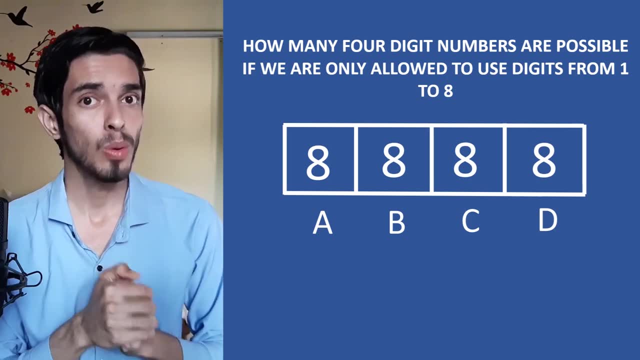 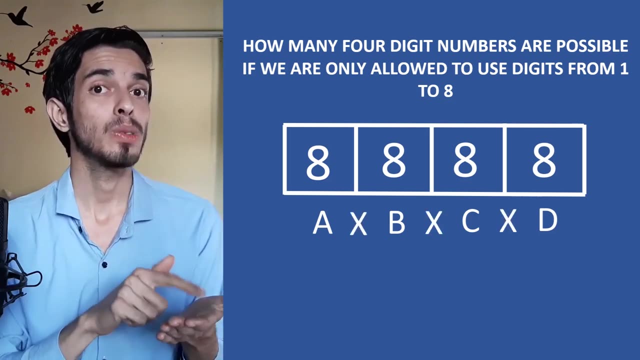 the second part, c- number of ways to do the third part and d- number of ways to do the fourth part. so here we will use the rule of products. so the number of ways to construct a four digit number, if we are only allowed to use digits from 1 to 8, is 8 into 8, into 8, into 8, which is 8, raise to the. 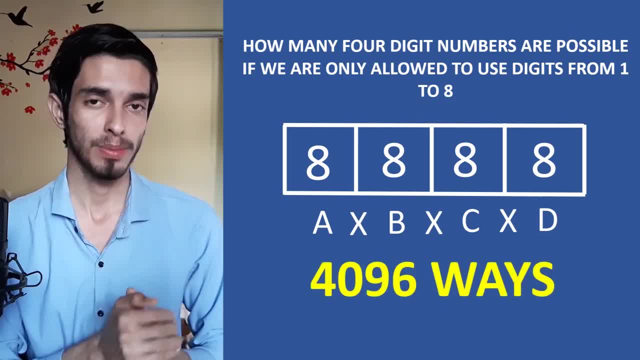 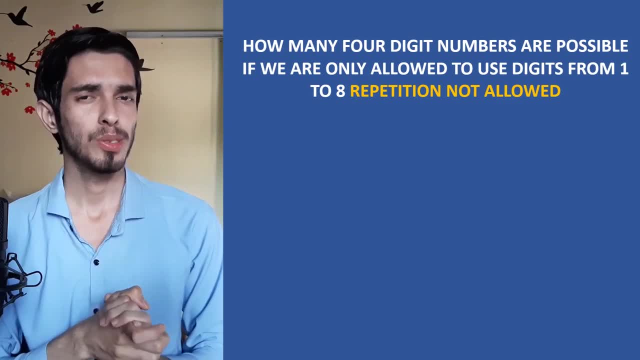 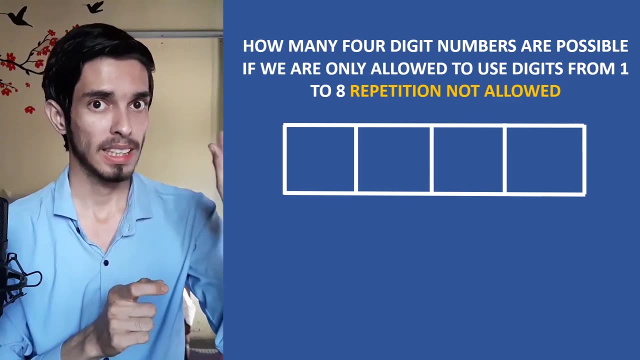 power 4.. so this is our answer to this question. now what happens? if the question says that the repetition of digits is not allowed, then what we will do. it's really simple: first try it yourself first. now see the number of ways in which we can do. the first part of this work is 8. now we have 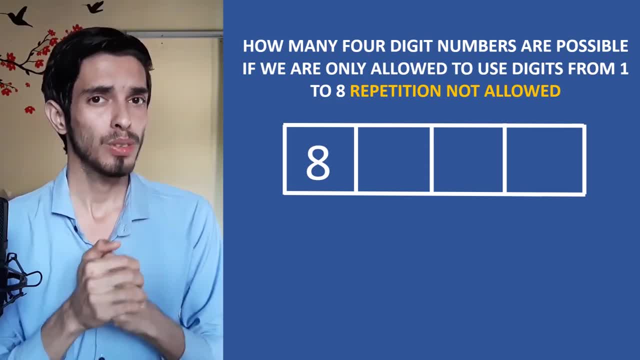 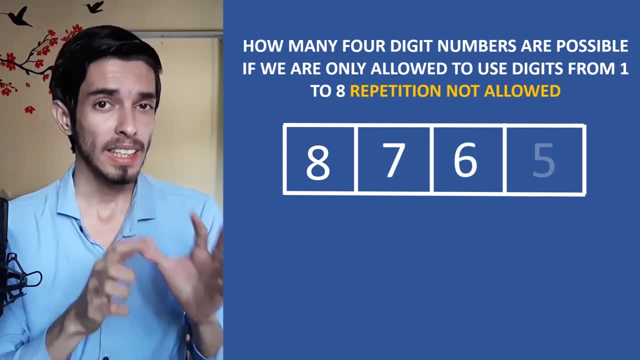 used one digit, so we can't use it another time. so now the number of ways in which we can do the second part of this work is 7, and so on 6, and so on 5, and here we are going to use the rule of. 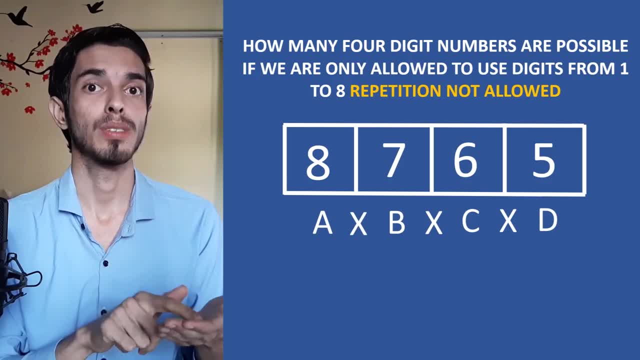 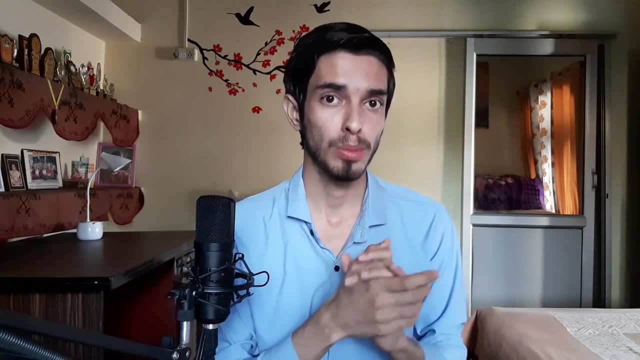 products. so 8 times 7 times 6 times 5.. so this is our answer. now let's just modify this thing a little bit to teach you another really important part of counting. now let us say you need to construct a five digit number and you are only allowed to use digits from: 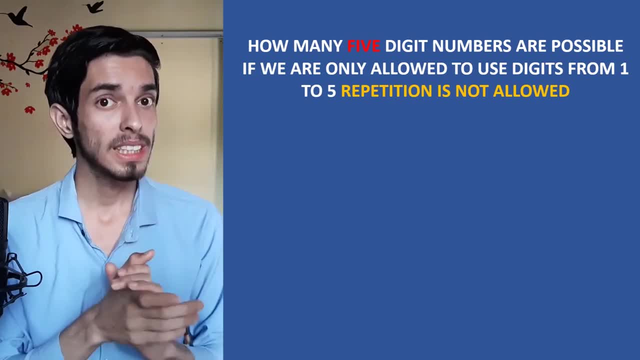 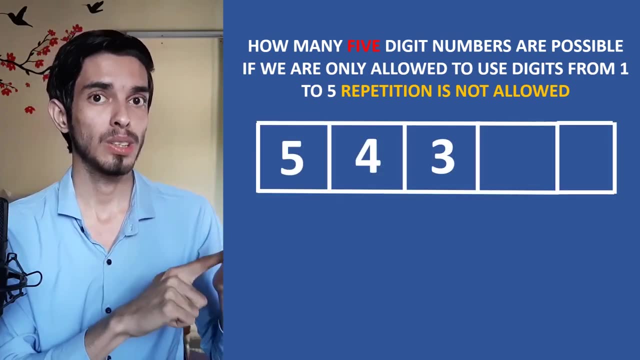 1 to 5 and the repetition of digits is not allowed. so the number of ways in which you can construct digits is 5 into 4, into 3, 2 into 1. okay, so what this thing is: 5 into 4, into 3, into 2, into 1. it is. 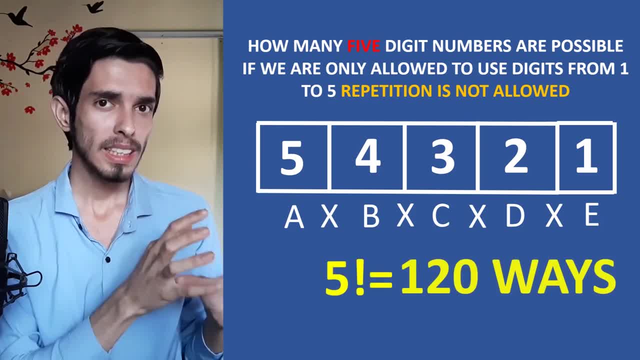 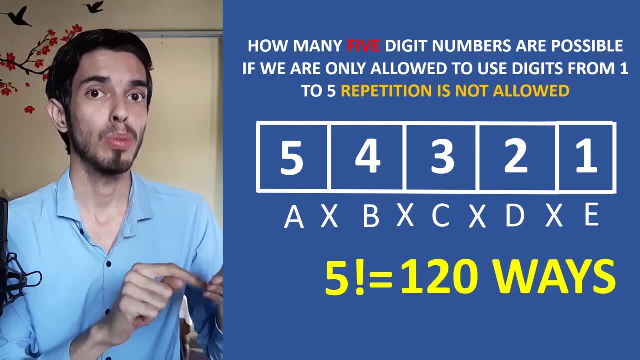 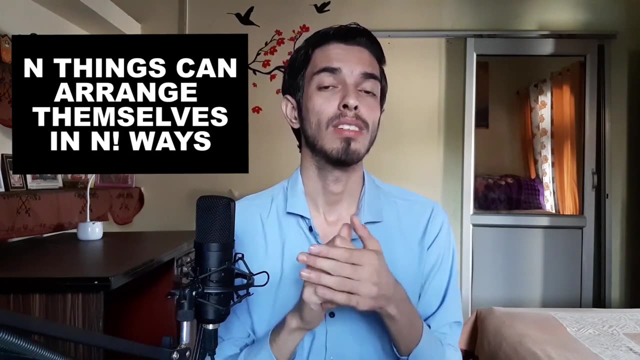 known as 5 factorial. so the answer is basically the number of ways in which 5 is allowed to be digits can arrange themselves in five boxes. so listen to this line very carefully: n things can arrange themselves in n factorial ways. okay, so this is really important and see repetition was. 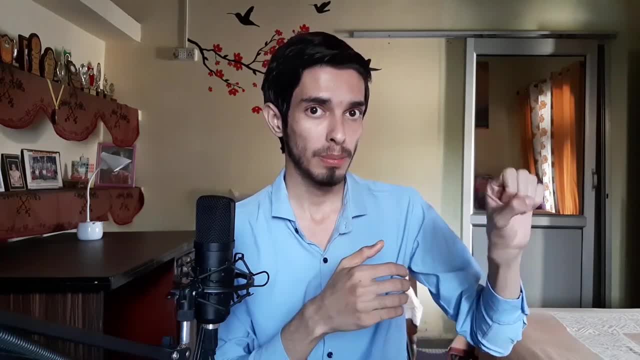 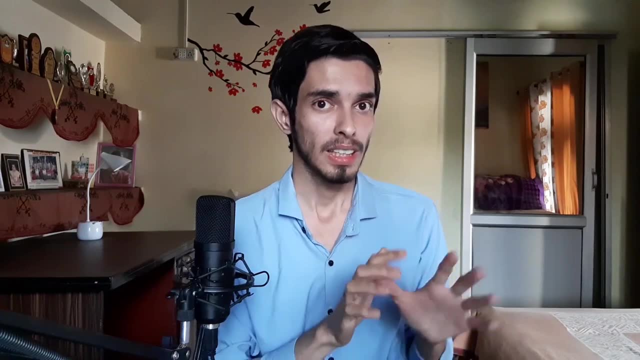 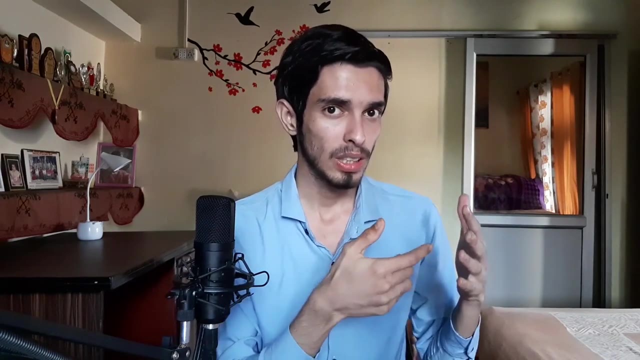 not allowed and that's why we were saying arrange themselves, because we are picking one thing and putting it in here. if repetition was allowed, it will be 5 raised to the power 5, and that is not arrangement. so n things can arrange themselves in n factorial ways and n factorial is basically. 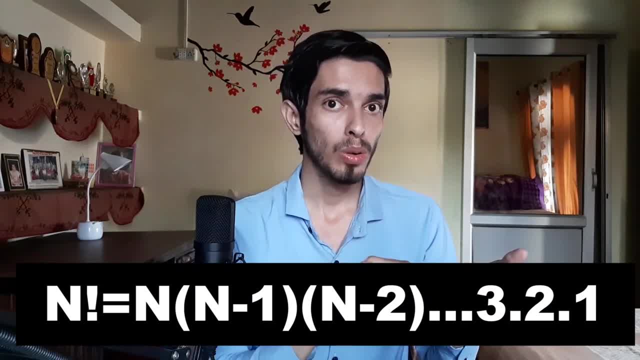 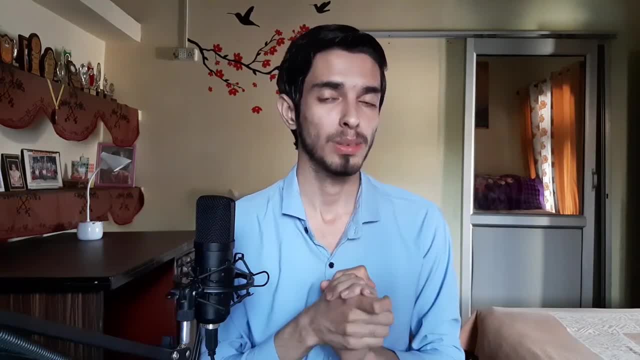 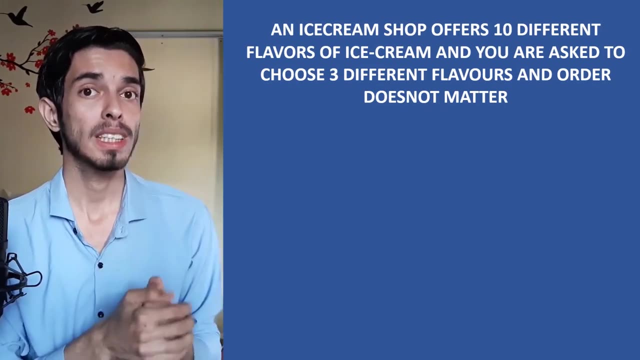 n into n minus 1, n minus 2 and so on to 3 to 1. so this is the definition of factorial and the use of factorial is really important to solve counting problems. now using this, let us solve another counting problem question now. the question is: an ice cream shop offers 10 different flavors of ice. 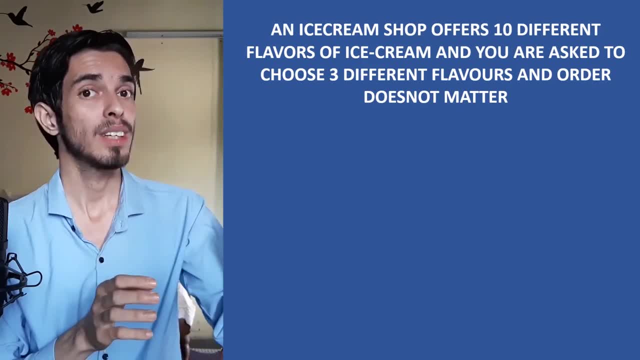 cream and you are asked to choose three different flavors of ice cream. and you are asked to choose three different flavors of ice cream. and you are asked to choose three different flavors of ice cream from them, and in here order does not matter. for example, you have an ice cream cone, you first. 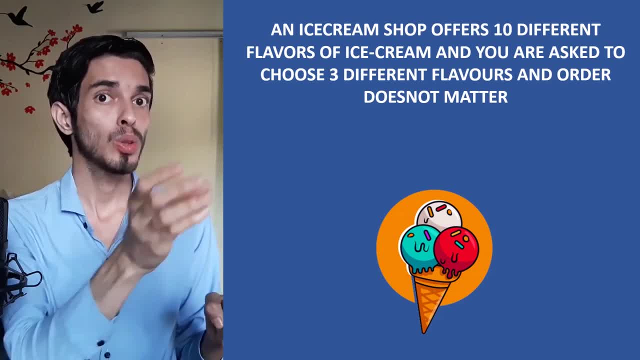 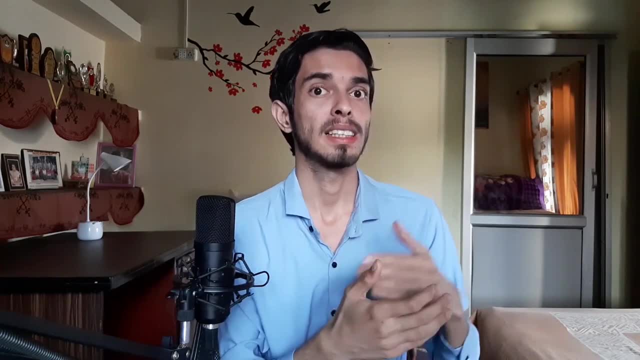 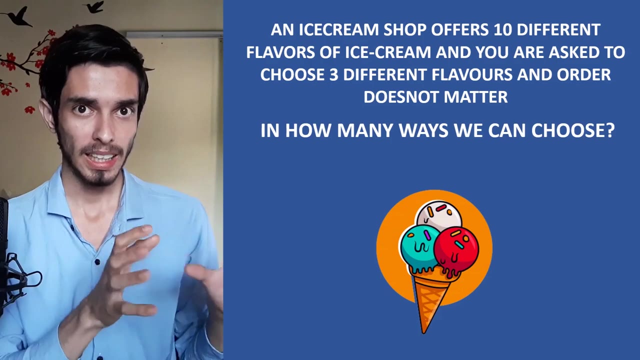 chose chocolate, and then you chose vanilla and then you chose mango. now, another time, you chose first mango, then vanilla and then chocolate. so this is not considered as a different choice. so the question is in how many ways you can choose these three different flavors. so in here see. 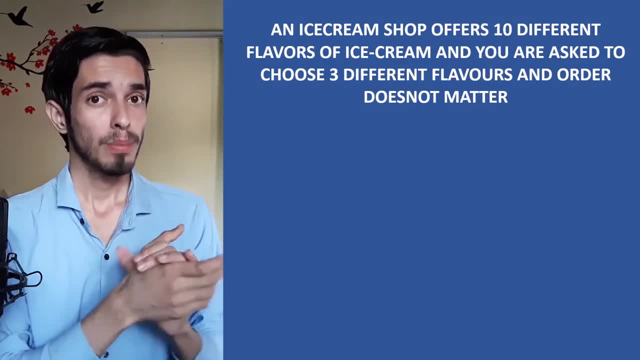 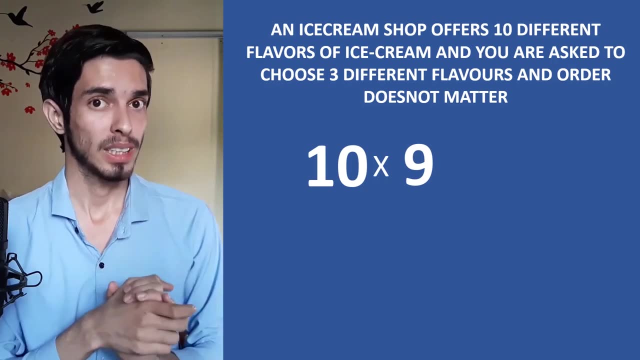 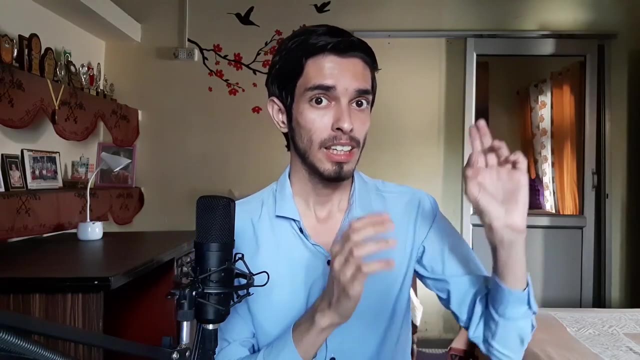 repetition is not allowed. okay, first thing. so the number of ways to choose the first flavor is 10, the number of ways to choose the second flavor is 9 and the number of ways to choose the third flavor is 8. okay, so is this our answer? no see, we have chosen three flavors, but we have over counted. 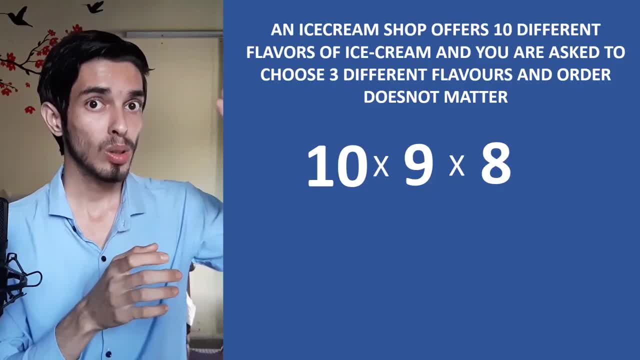 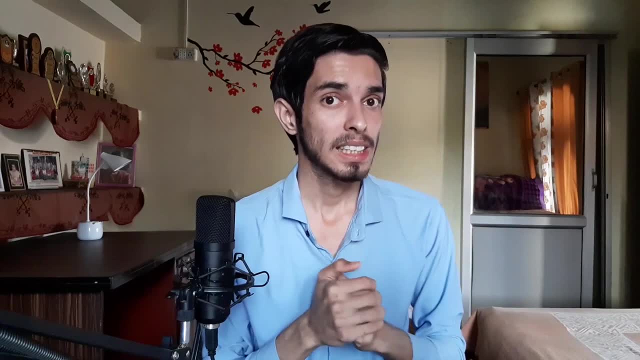 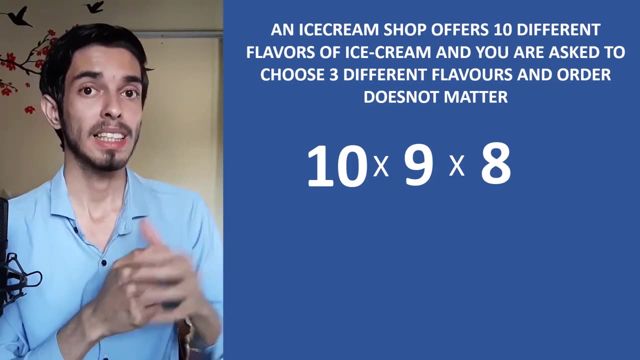 because the order did not matter. so in here we are also counting the arrangement of these three flavors. we need to reduce it. so three flavors can arrange themselves in three factorial ways, which is three to one, 9 into 8, divided by 3, into 2, into 1.. Okay, so this is our answer. Now, factorials are really. 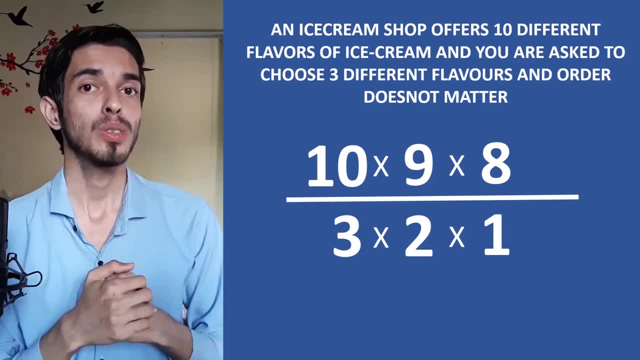 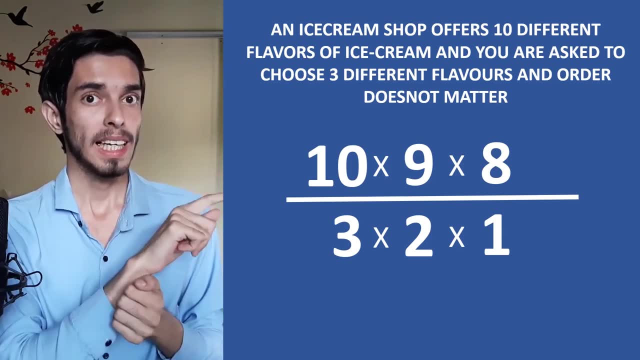 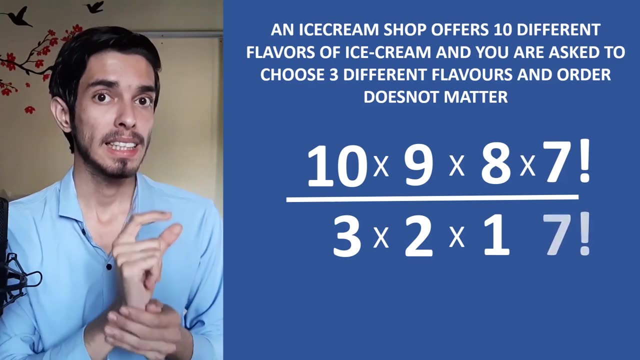 important in counting problems, So we need to convert this into factorial. So see, we can write this as 10 factorial divided by 7 factorial, because see 10,, 9,, 8 and there will be a 7 factorial, So 7 factorial will get cancelled with it. So we have just multiplied and divided it by 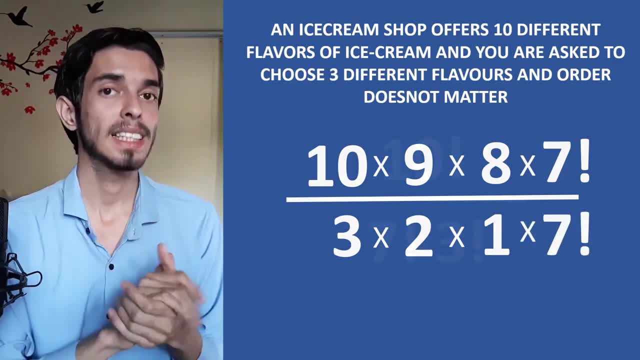 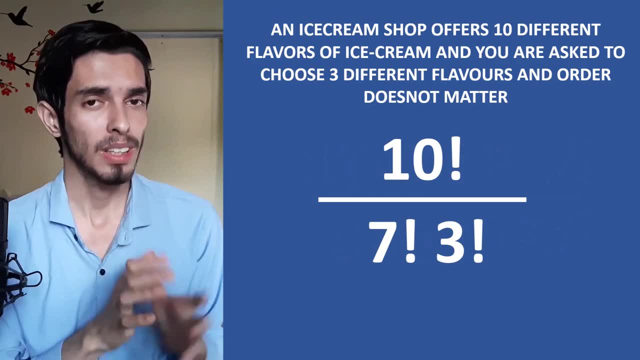 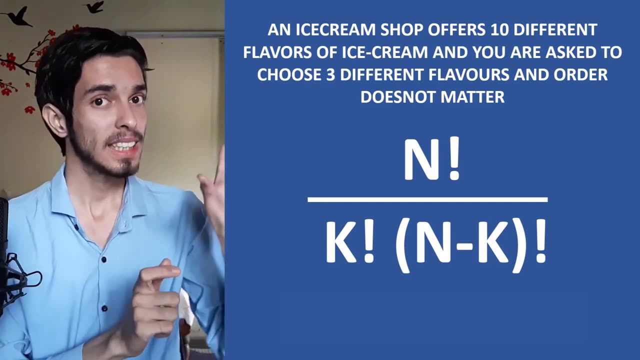 7 factorial and we can write the above one total as 10 factorial. So we have 10 factorial divided by 7 factorial multiplied by 3 factorial, So we can write it as N factorial divided by k factorial, N minus k factorial. and this is basically the formula for combination which is written as N. 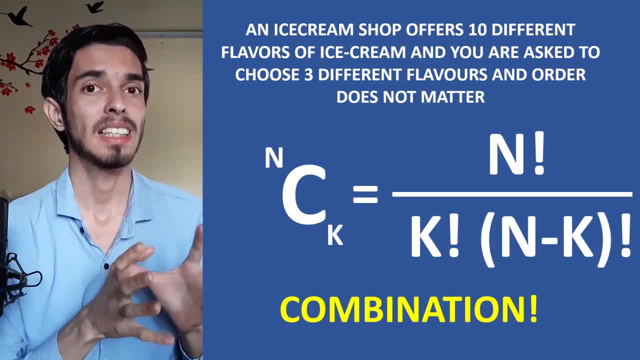 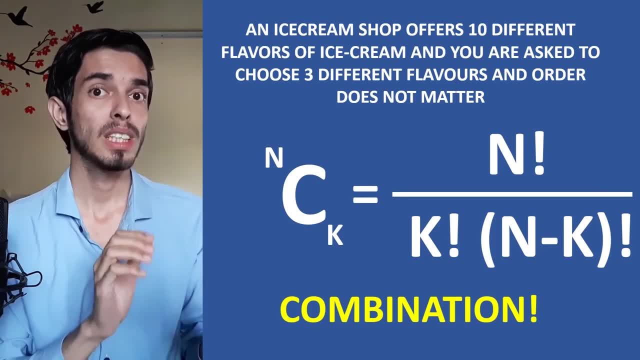 c, k. So this formula of combination is another really important thing in counting problems. So we read it as Nck n choose k, and this is used where we need to choose k things from n things, and the order in which we choose the k things does not matter. So this is really important. you need to remember this. 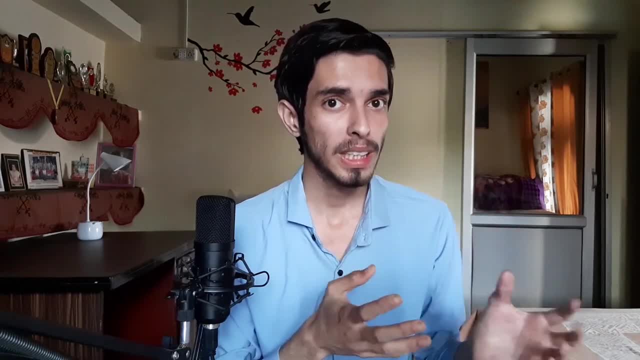 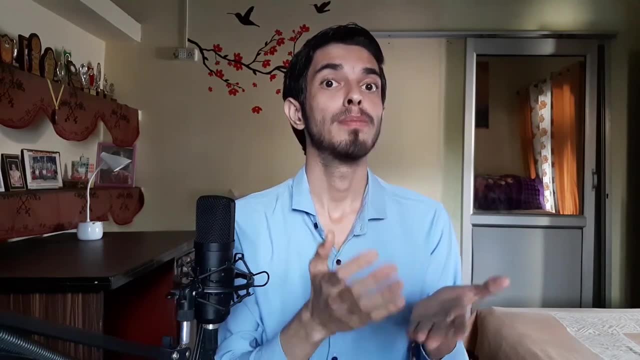 formula. Now the second really important formula is the formula for permutation. This is similar to combination, but in here we will choose k things, but in those k things the order matters in here. So in here the order matters, so that 3 factorial won't come in here. so we will remove that 3. 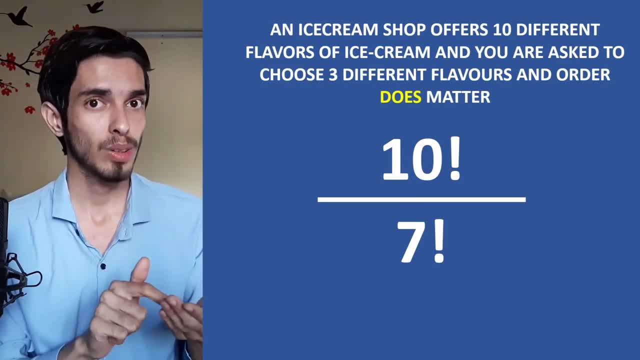 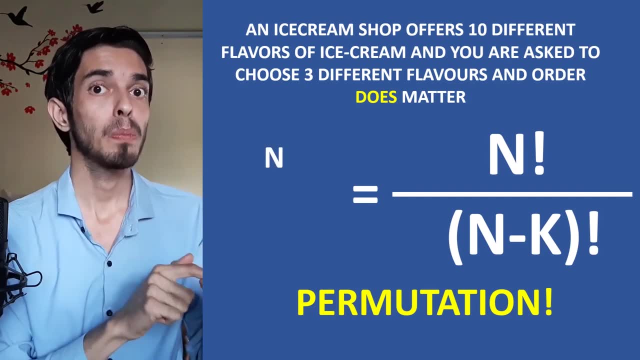 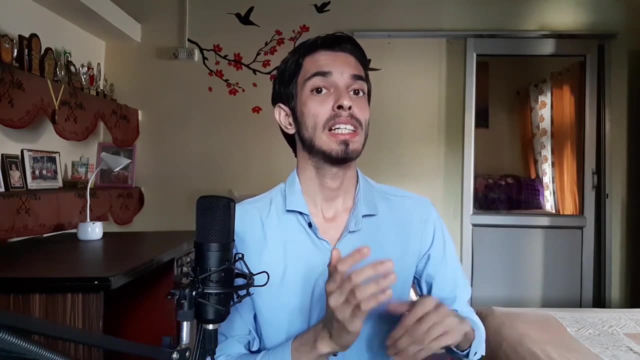 factorial. So in here we have 10 factorial divided by 7 factorial and we can write it as n factorial divided by n minus k factorial, which is written as np3, and p stands for permutations. So combinations and permutations are basically another name for counting problems. So in most math textbooks the 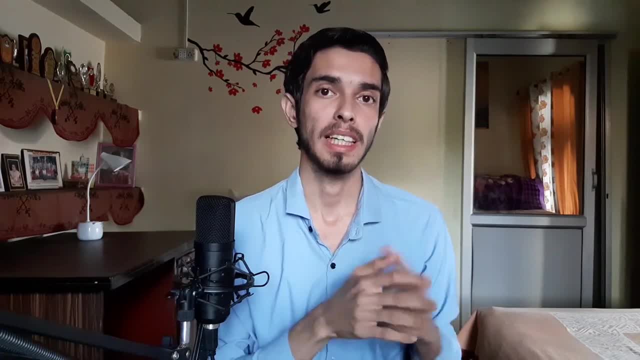 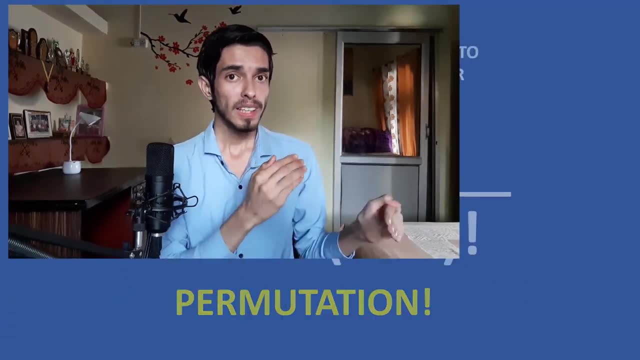 counting problems are there in the permutations. So in most math textbooks the counting problems- permutation and combination- named chapter. Why I am telling you this? because you can go there and try out some counting problems after watching this video. Now let us say you had another shop in which 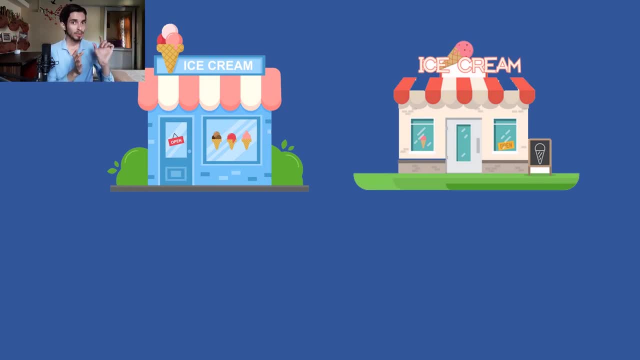 there are 10 different flavors, okay, but at the same time you can only take one ice cream. So the number of ways in which we can choose from both these two shops is basically the number of ways in which we can choose the first shop plus the number of ways in which we can choose from the.